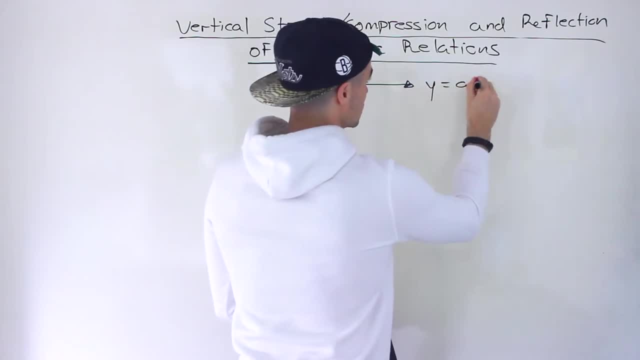 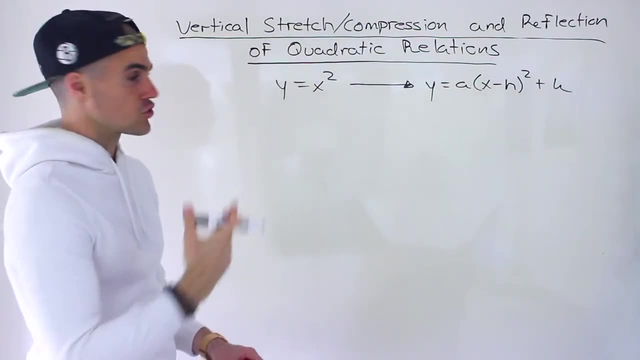 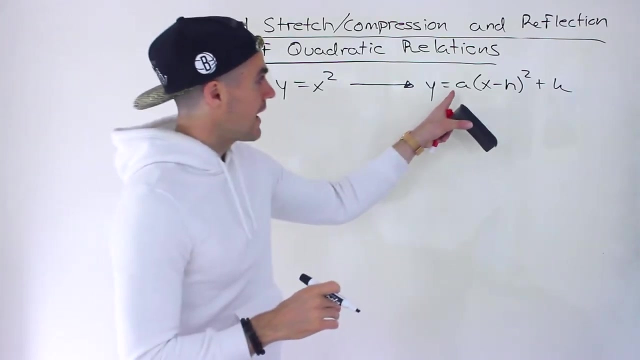 we're going to specifically be looking at in this section is that vertex form? Okay, that's where that's the kind of format that gets outputted once a quadratic goes through certain transformations. However, I also mentioned that the a, h and k value, those are what's going to affect the transformations, depending on what 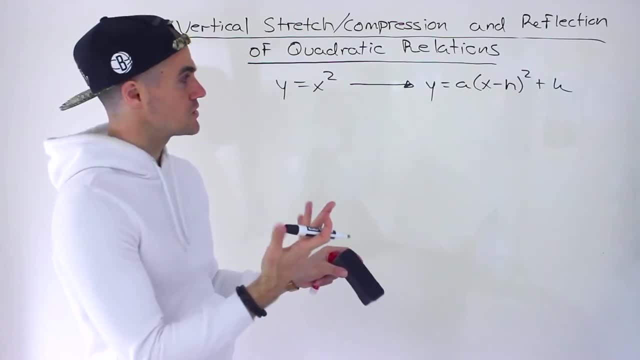 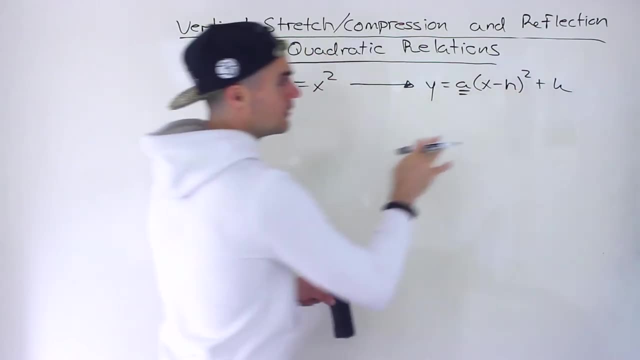 values those take, but we're going to go through them one by one. I mentioned that as well. so in this particular video, what we're going to do is we're going to focus on the a value, So we're going to just pretend that the h is zero, the k is zero, we're going to forget about those, and so. 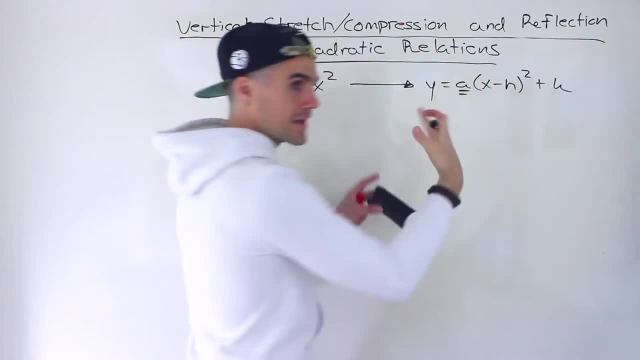 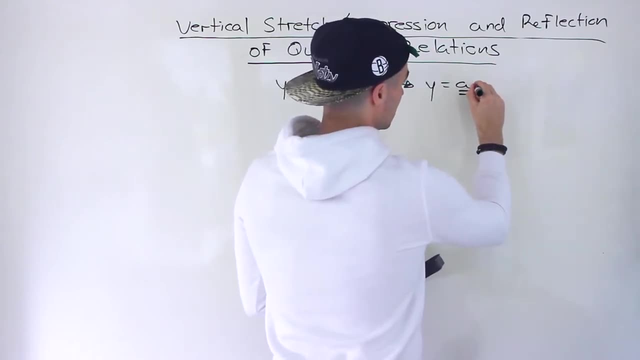 instead of looking at this entire format where we're mixing all the different transformations. we'll be doing that in the future. Here, in this particular video, we're going to focus on the a value, so we're going to just pretend that the particular video we'll just be looking at that a value. How does that a value affect that base? 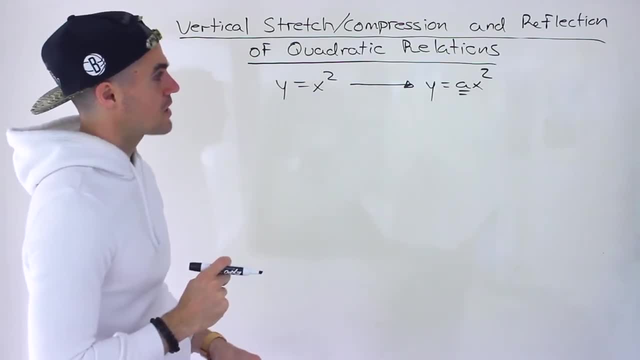 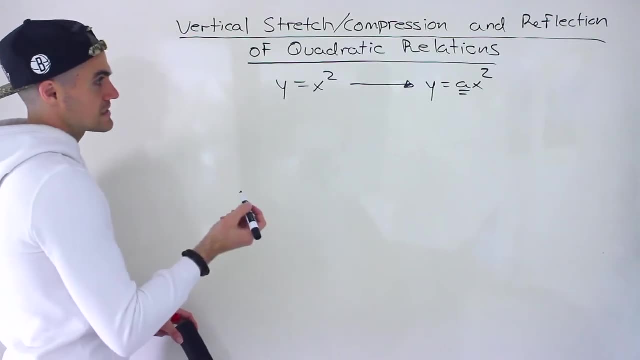 function. y equals x squared and it really depends on the value that the a can take. So there's different values. so here are the different cases that can happen. We can have an, a value that is greater than one. that's the first type of case and if this happens over here, if a is greater than 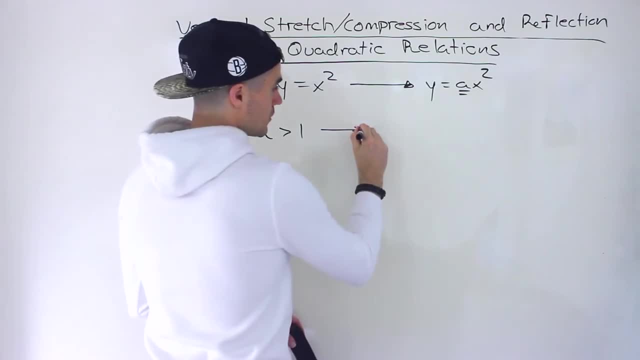 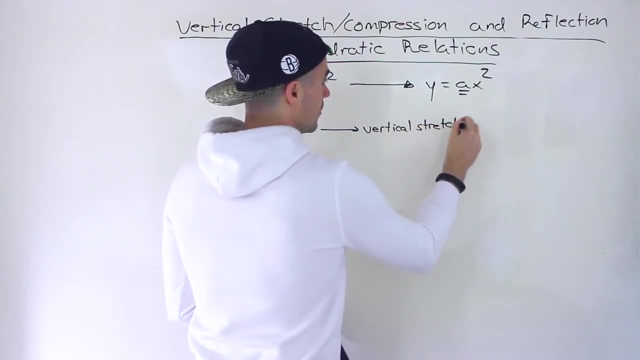 one, that's the first type of case. and if this happens over here, if a is greater than one, that's the first type of case. and if this happens over here, if a is greater than one, that's the first type of case. then what the transformation is going to be is there's going to be a vertical stretch. 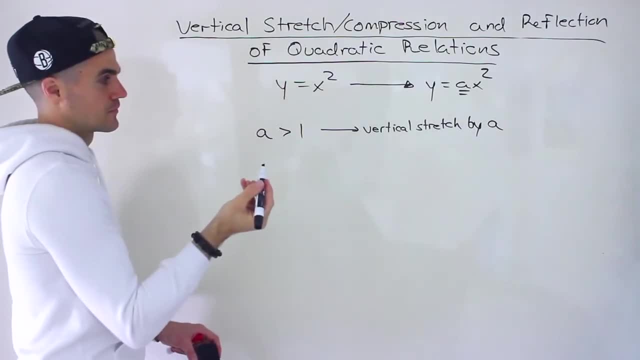 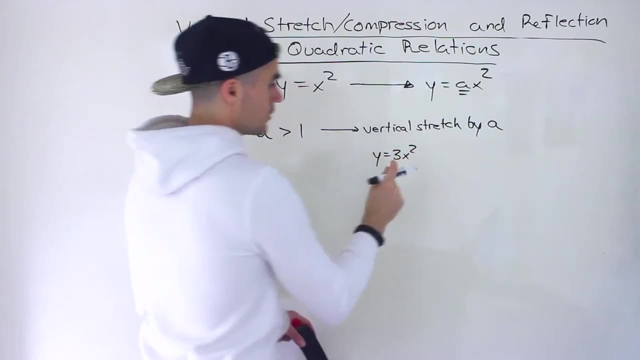 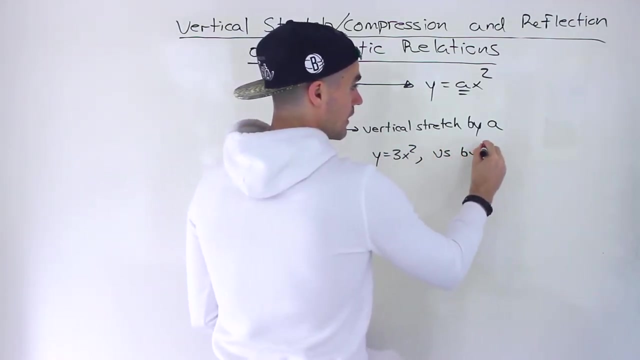 by a factor of a. So, for example, if we have, like the function y equals 3x squared right, notice that the a value is greater than one, the a value is three. in this case this: here there would be a vertical stretch by a factor of three. 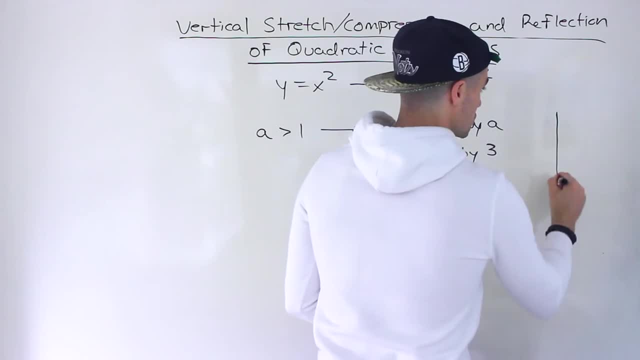 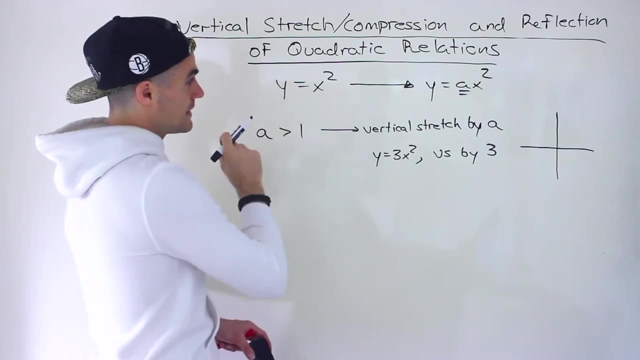 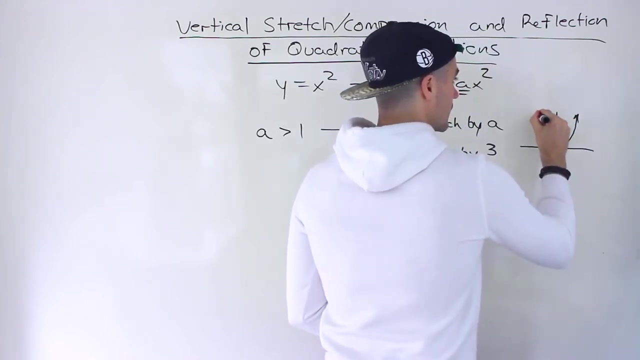 Now the way this looks graphically. in each of these cases, I'm going to show you how this kind of function with an, a value greater than one, relates to the function x squared. So let's say that we have x squared like this, right? so this here is x squared. Let me show you in a 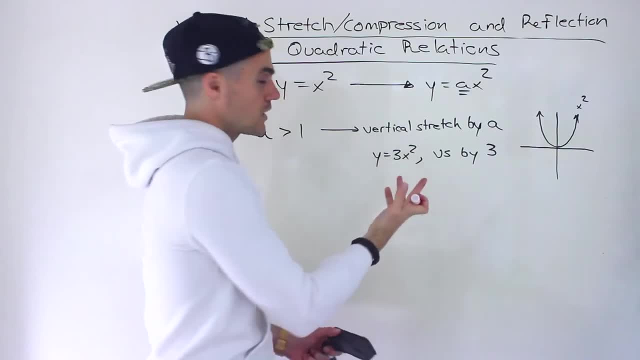 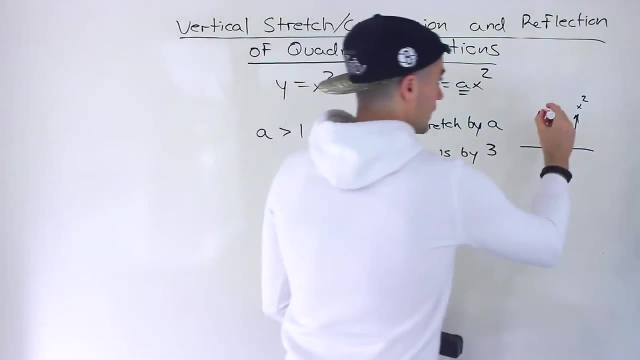 different color. the way, for example, y equals 3x squared is going to look, or any a value that's greater than one could be 2x squared, 5x squared, 10x squared. whatever it's going to look, something like this: okay, it's going to be. 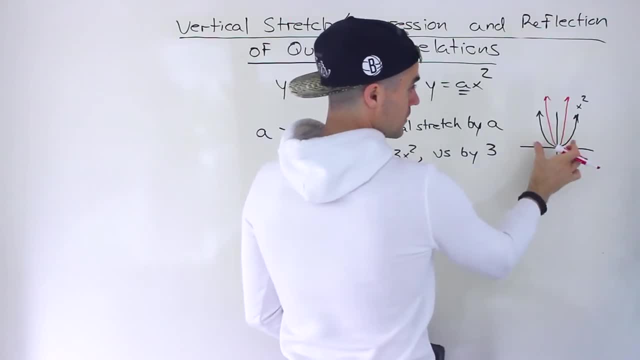 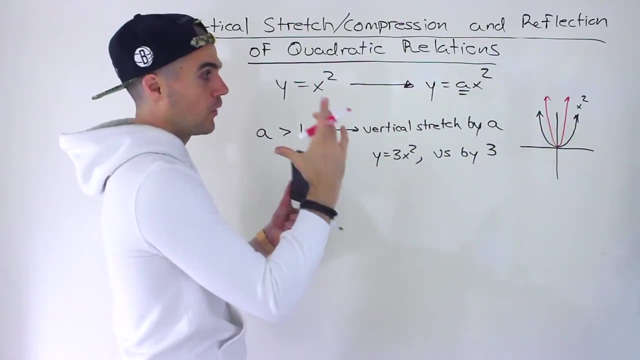 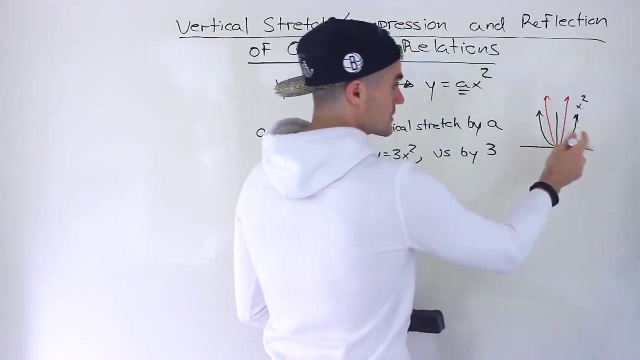 vertically stretched right. so if this is x squared right, if you plot x squared, for example, if you go to decimals, plot one graph x squared and then another graph you plot 3x squared, or 5x squared, 2x squared, that graph is going to look like this in relation to that: 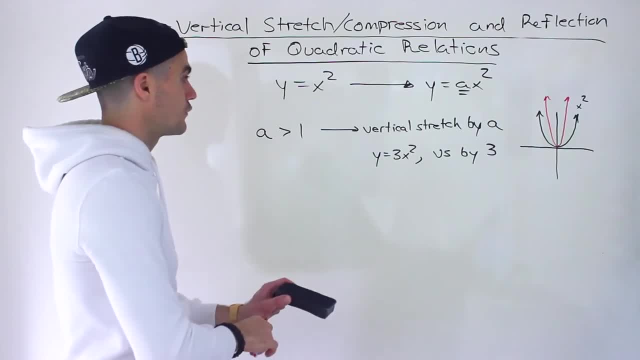 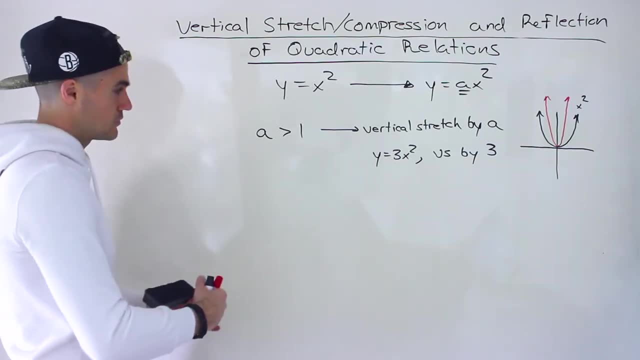 x squared graph. So that is the the first case. so if an, a value is greater than one, there's a vertical stretch by a factor of that a value. Now the next case is if a is equal to one. and if a is equal to one, let's sort of split these up here. if a is equal to one- well, notice what are we just? 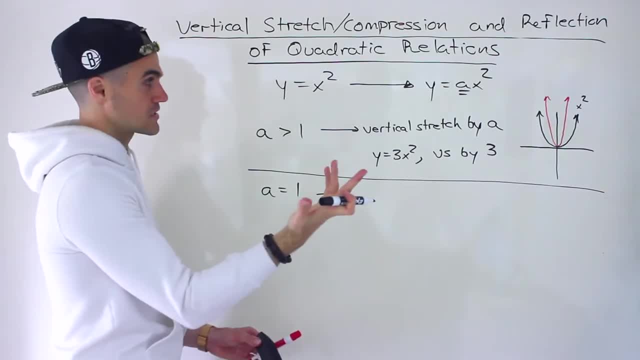 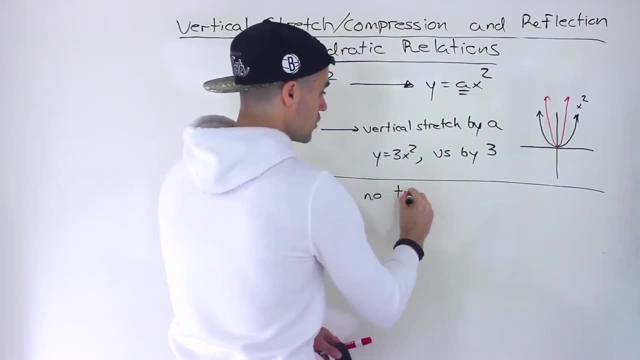 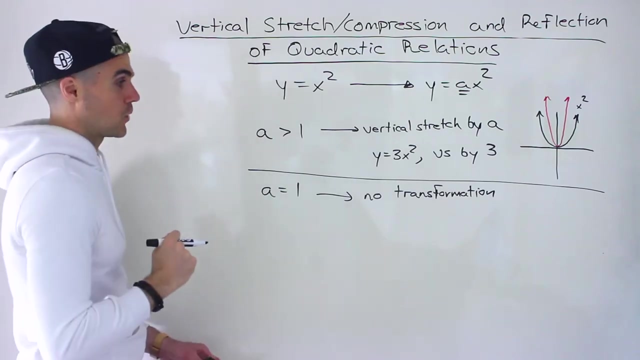 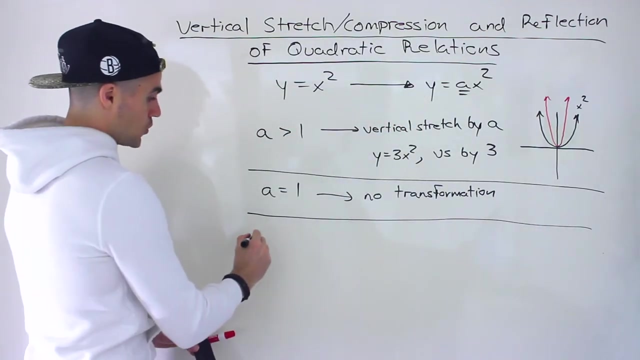 going to get. we're going to end up with that same function: y equals x squared- right, there will be a, so an a value of one means that actually there's no transformation, right? it's just that same base or parent function: y equals x squared. The next case is if a is between zero and one. 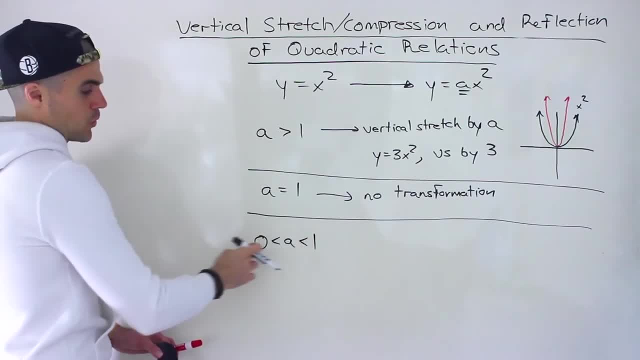 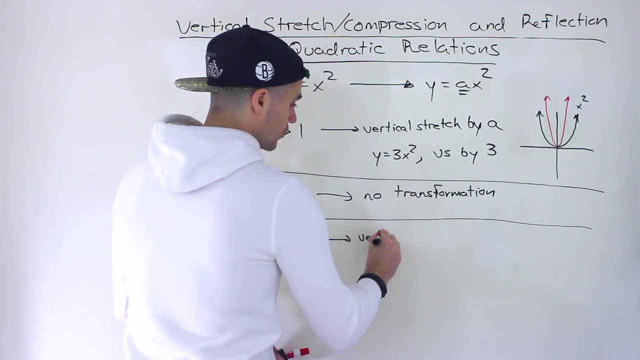 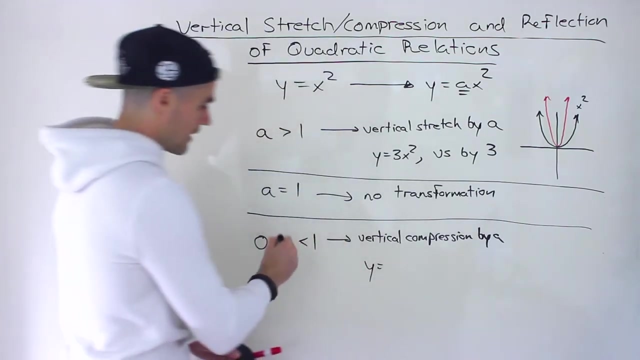 okay, if a is between zero and one. if that happens, then we're going to have a vertical compression by a factor of a. okay, so an example of this would be like: if we have lots of times these a values here between zero and one, they could be decimals, so maybe like 0.5. 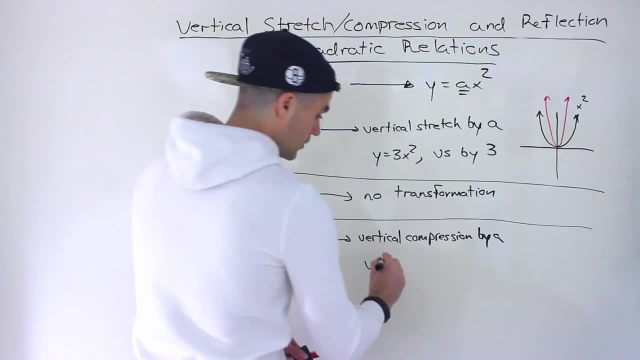 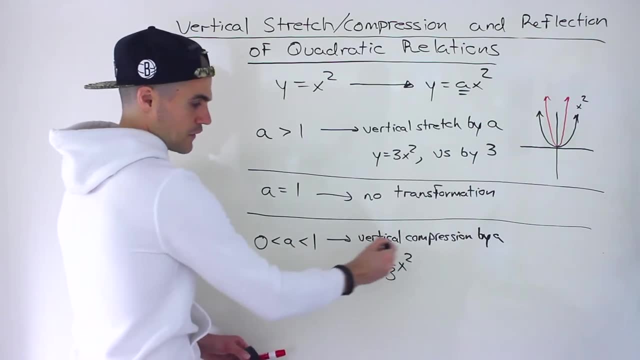 x squared or 0.2 x squared. a lot of times they'll be fractions as well. so let's put a fraction. let's say it's like one over three x squared, like that. if you get a function like this, they ask you to state the transformations that are undergone on x squared. here you would say there's. 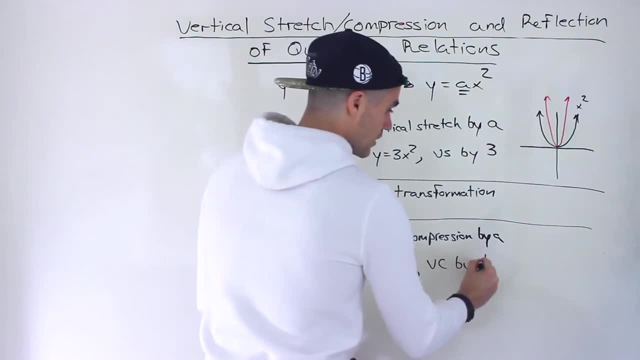 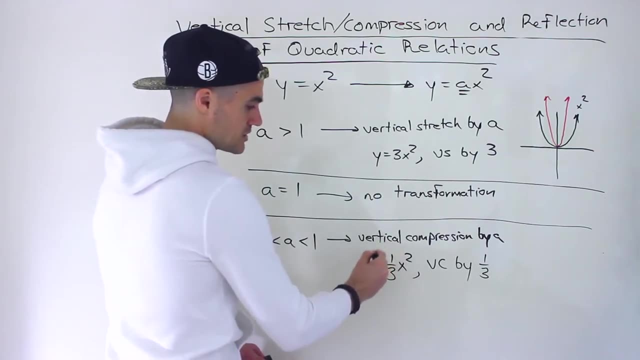 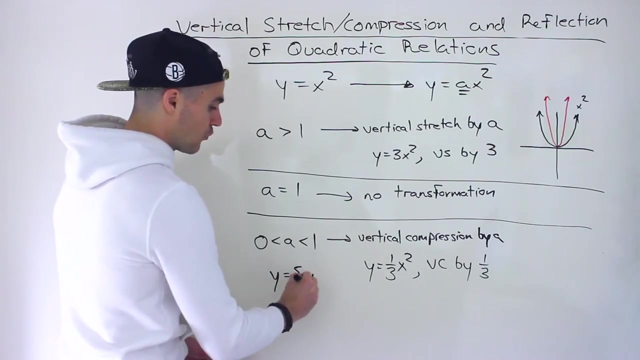 a vertical compression by that same factor of one over three. now just one thing I want to mention. you want to be careful here. not all fractions are necessarily a vertical compression. so, for example, we can have y equals, let's say five over four, x squared. notice that this is a fraction. but if you 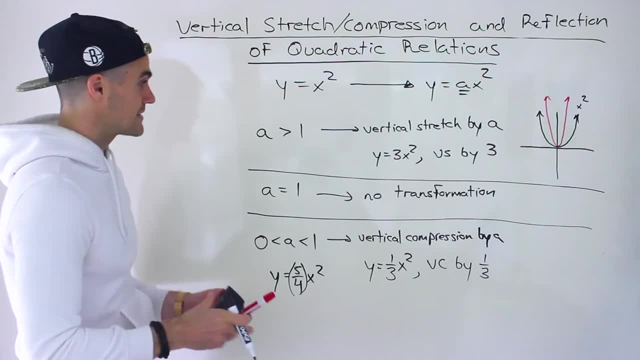 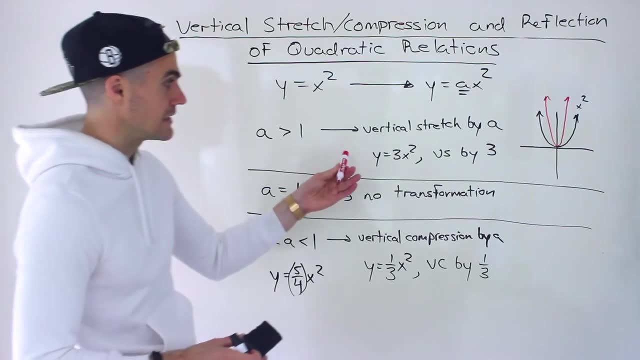 look at the. a value five over four is one point two five. so that's a fraction of one over three, that's an a value greater than one, and so this particular function, this particular quadratic would actually be in this case. so this would be a vertical stretch over here. but if it would be, 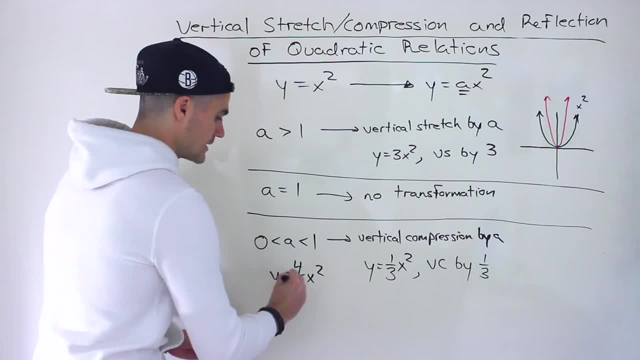 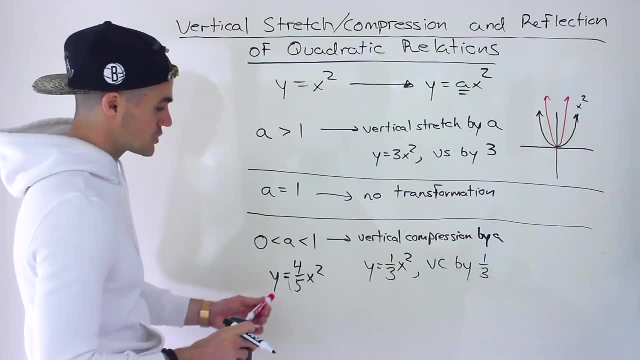 let's say four over five. right, that's 0.8. that would be a vertical compression by four over five. so just be careful. lots of times students will see fractions and then they'll automatically assume that it's this case, because a lot of times this a value is greater than one, and so this particular 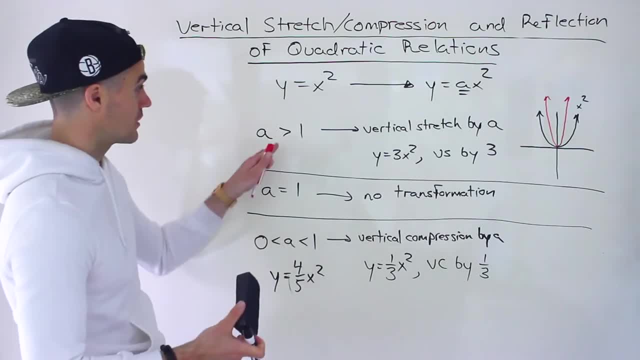 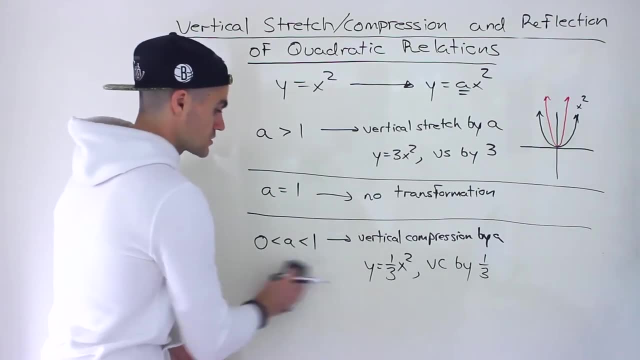 value between zero and one is given as a fraction, but some fractions can also be greater than one and they would end up being a vertical stretch and not a compression. so just be careful with these fractions. so this will either be a fraction or a decimal to represent an, a value between zero. 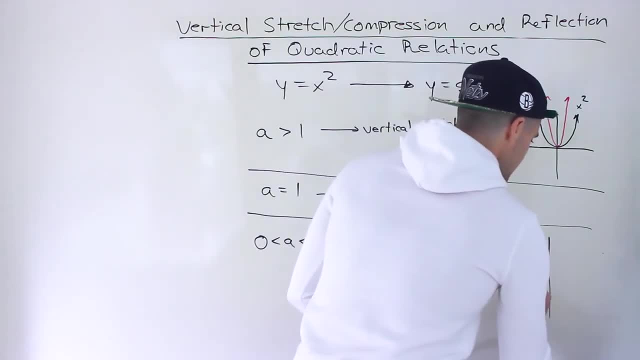 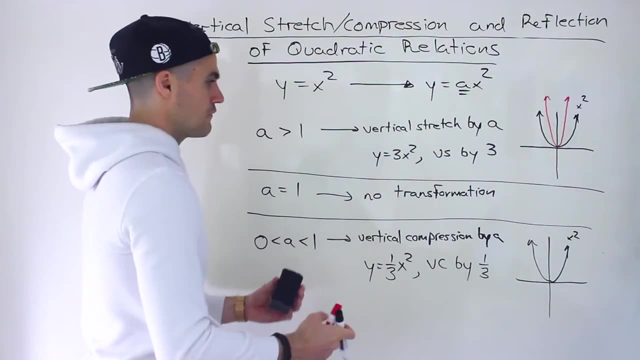 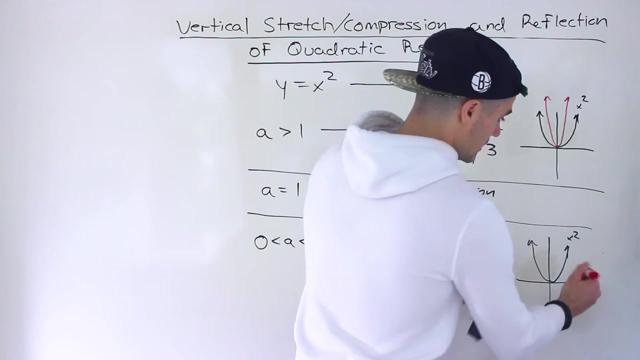 and one. now the way this looks graphically. again, let's say that we have the base function x squared like this: if we end up having a function with an, a value between zero and one, it's going to be vertically compressed, okay, so what that would mean is that the function would 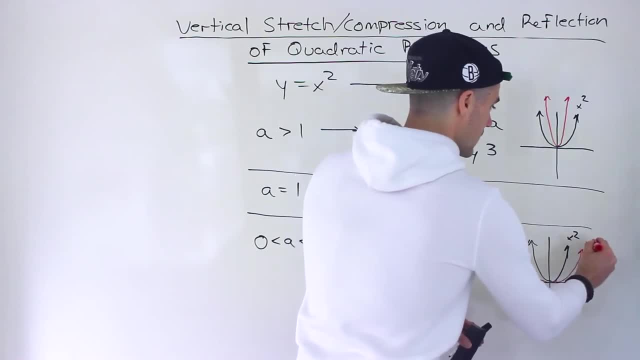 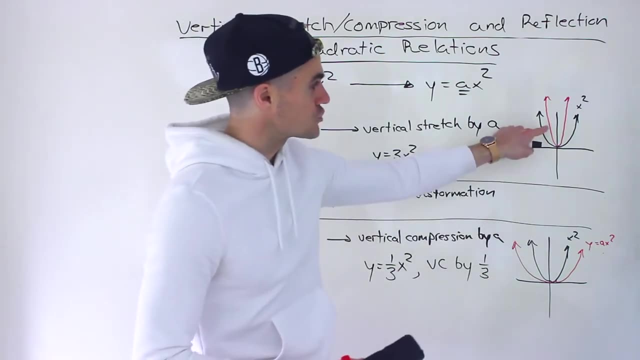 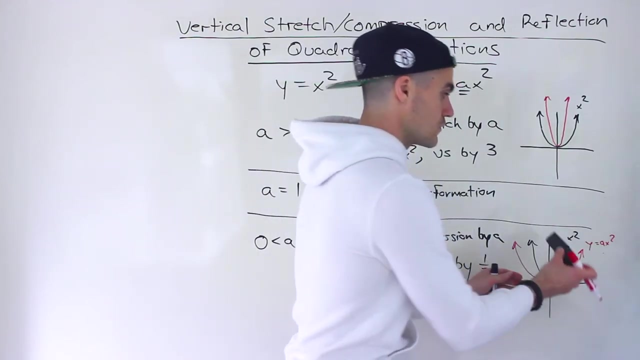 end up looking like this: y equals ax squared, and that's if a is between zero and one. so notice the difference between a vertical stretch- that's how a function looks like- and a vertical compression. right, the function becomes wider. so if you go to desmos, if you plot x squared and then maybe like: 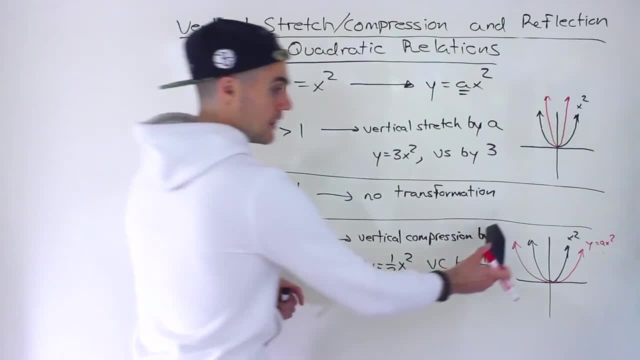 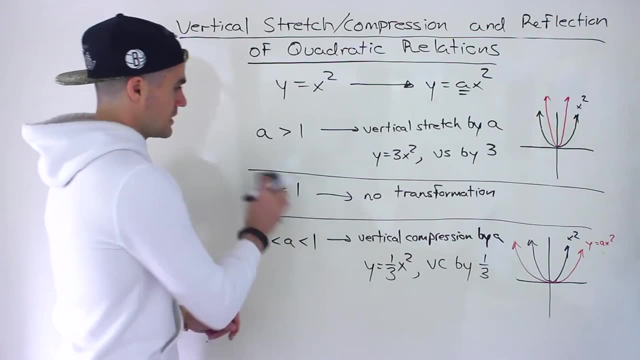 0.5 x squared or 0.1 x squared. it's going to be a vertical stretch and then it's going to be a x squared. that's how that transformed graph is going to look in relation to x squared. so, moving on with the uh, with the cases, let me actually erase it over here. what would be the next case? 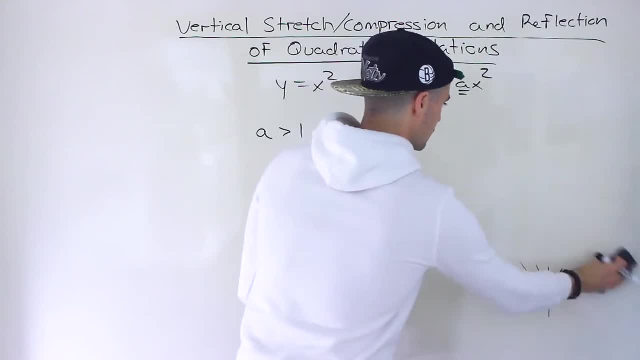 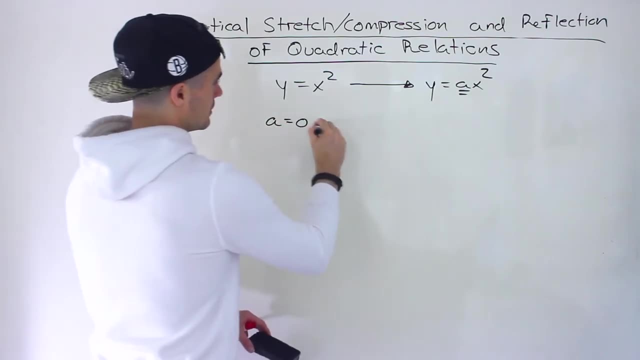 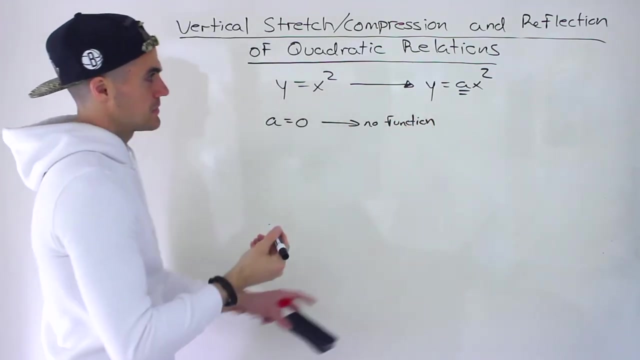 so the next case would be: if we have an a value of zero, right, an a value of zero would actually there would end up being no function, all right. so usually you're not going to get that case, because if a is zero, then we'll just end up having y is equal to zero. 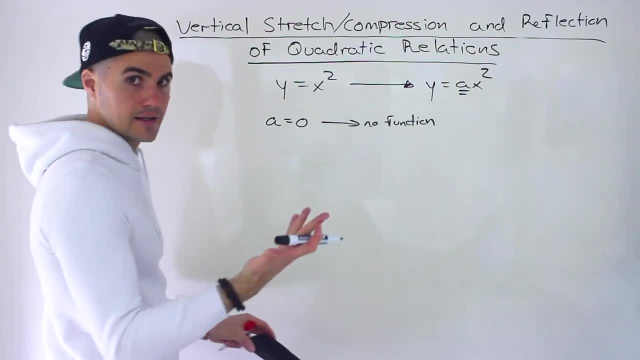 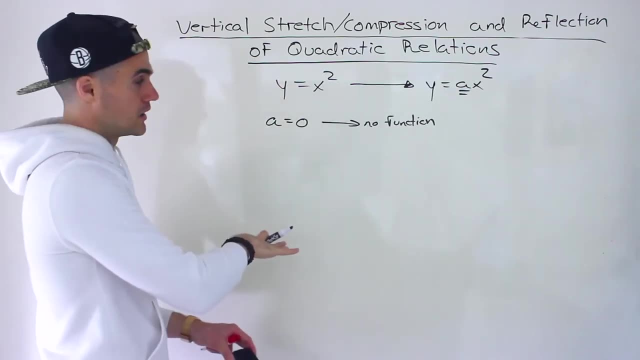 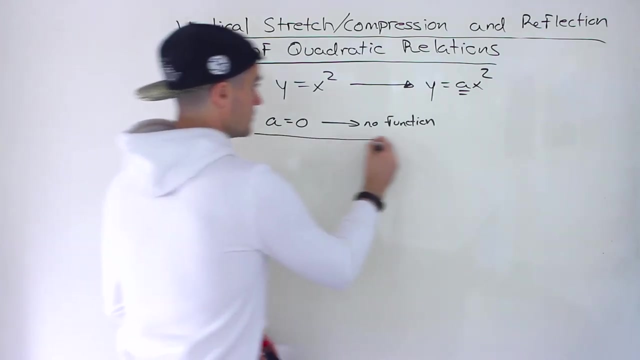 and that is just the horizontal line at a y value of zero, right? so this case you don't necessarily have to worry about. i'm just going through all the potential or all of the possible cases that can come up for a now. after zero, the next, if we're going in order, the next case would 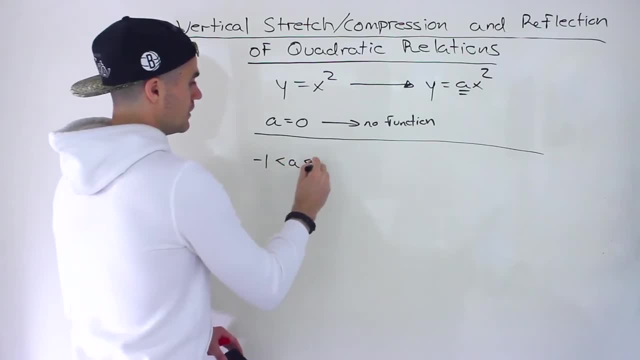 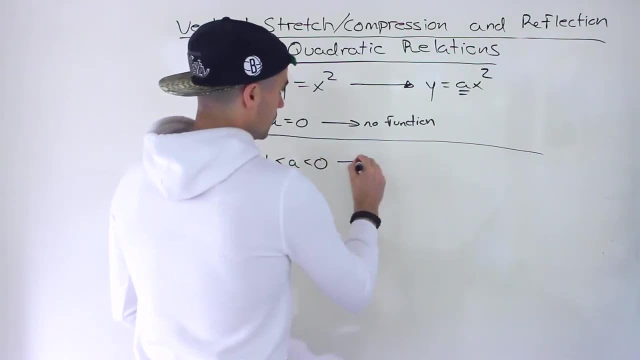 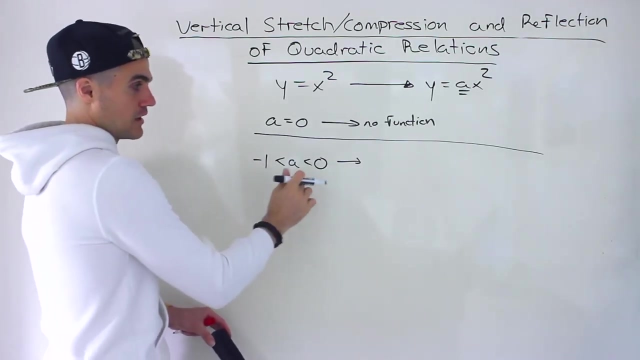 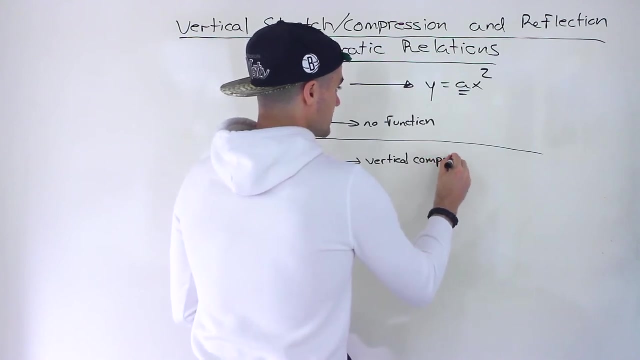 be. if a is between negative one and zero, and if this happens here, then we still have remember: when a is between zero and positive one, there was a vertical compression. well, if it's between negative one and zero, then there's also a vertical compression. however, what we do is the factor that we mentioned. it's compressed by 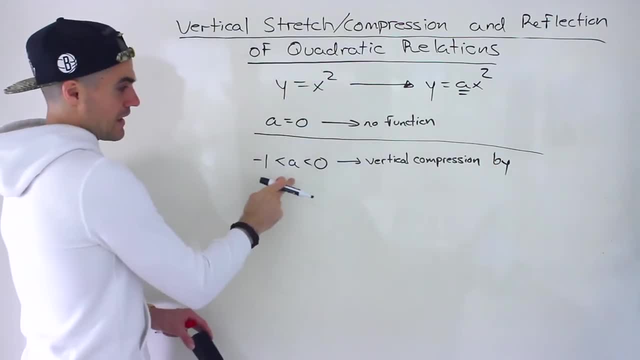 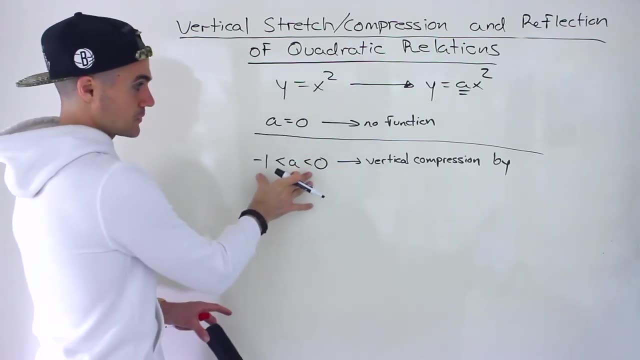 is not the negative a value. notice here: this is going to be a negative a value. right before we were dealing with the positive a values. now we're dealing with the negative a values. when we say it's vertically compressed, here we don't say by let's say let's. 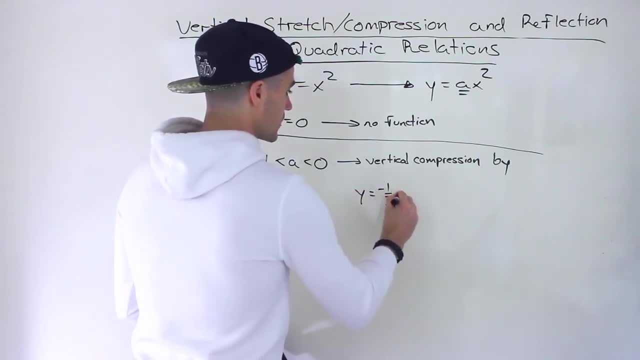 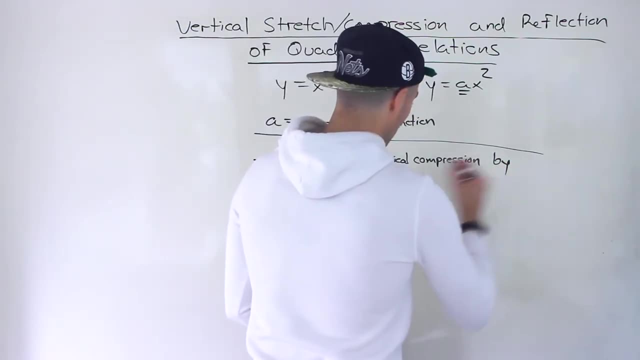 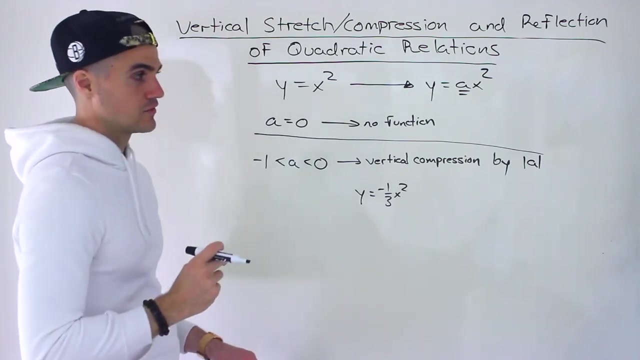 say we're dealing with like y equals negative, one over three, x squared. we don't say it is vertically compressed by negative, one over three. we still say it's vertically compressed by positive, one over three. and so the way that's represented here generally is, we say, by an absolute value of a. 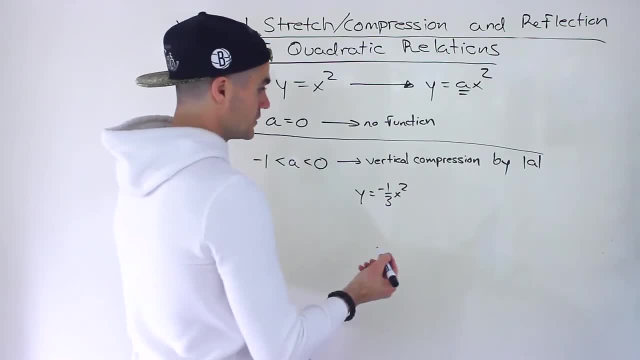 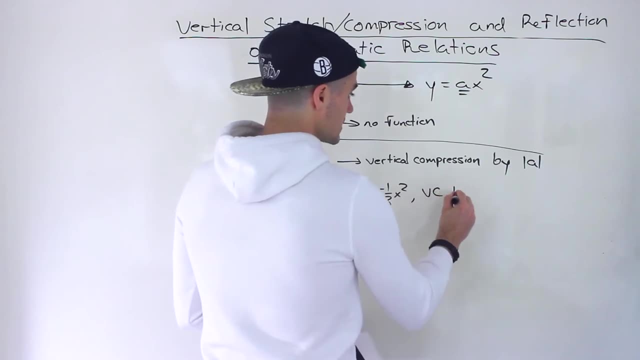 that's what the factor is going to be and what an absolute value does is. it takes any negative, turns it into a positive. so this here we would say it's vertically compressed by an absolute value of negative one over three, and so this here is just the same as one over three. right, don't get confused with this. 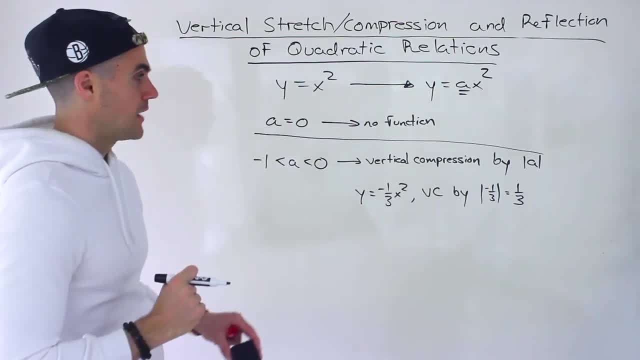 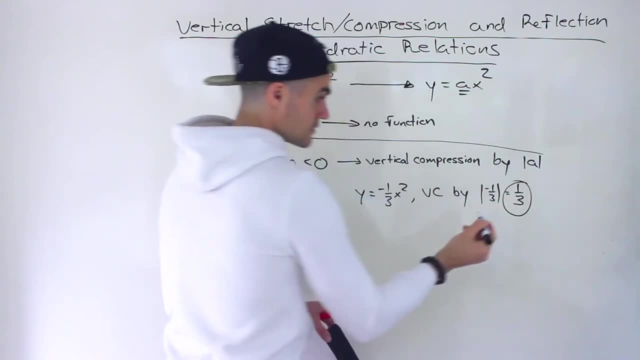 this absolute value. i'm just mentioning it because some textbooks may write a description like that. basically, if you get something like this, what you want to say it's vertically compressed by positive one over three- you don't want to add that negative when you're stating the factor the. 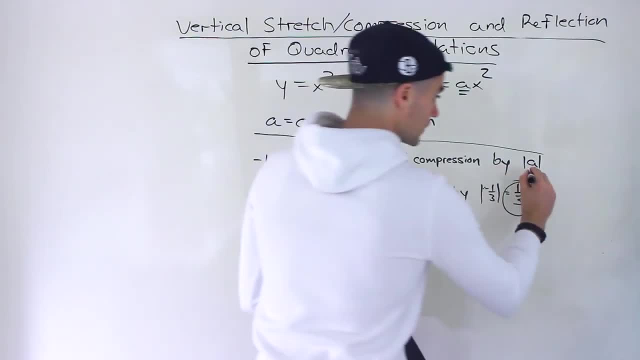 factor is always positive, so you may want to write a note here: this here is always positive. so then, what is the difference between if we have, for example, positive one over three or negative one over three, because when i was positive one over three, it was also vertically compressed. 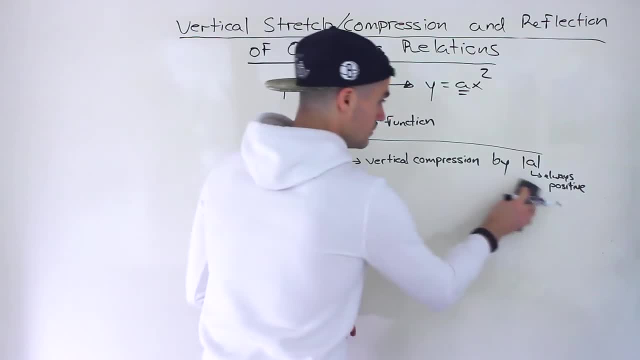 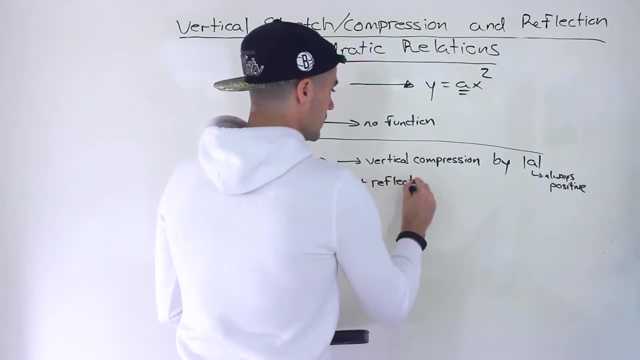 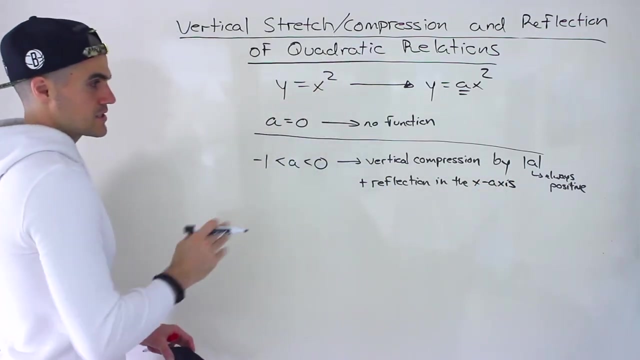 by one over three. well, if it's negative, there's also an additional transformation. there's also a reflection in the x-axis, right, so the x squared is going to be reflected. so now it's actually going to be opening downwards. so that's another thing, uh, to mention on the side here. if you have any positive. 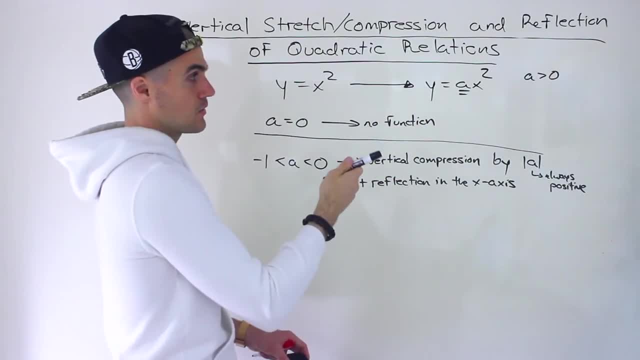 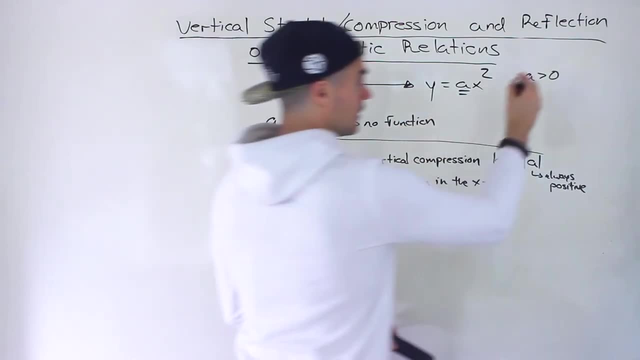 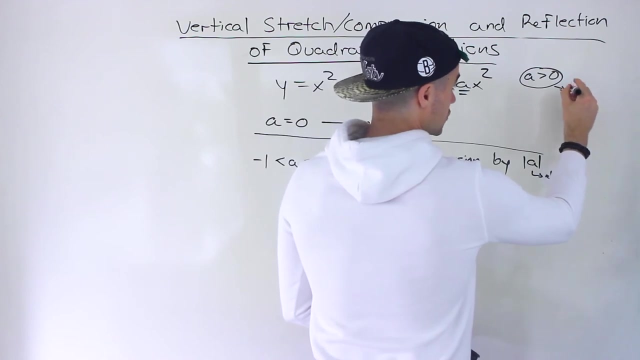 a values. uh, so that could be between zero and positive, one, one or greater than one or greater than one. all three of those first cases that we went over, for all of those a was greater than zero, it was positive, and what that means is that the quadratic is opening upwards. 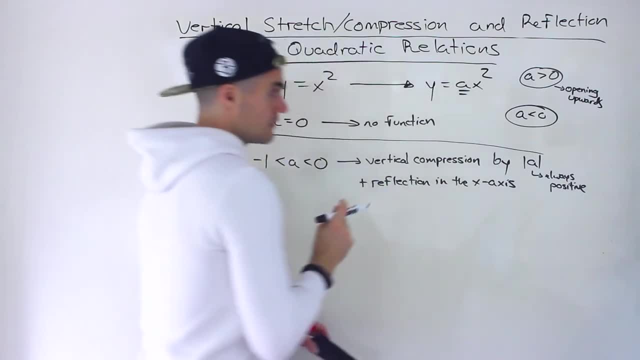 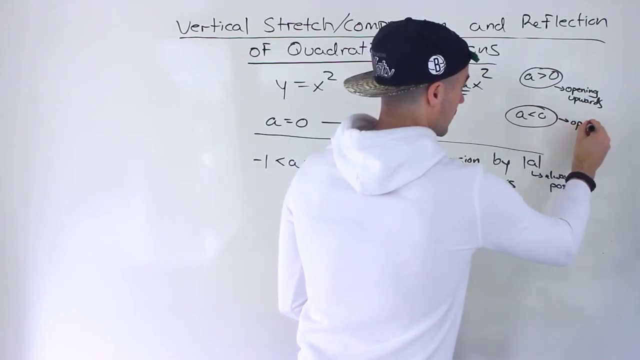 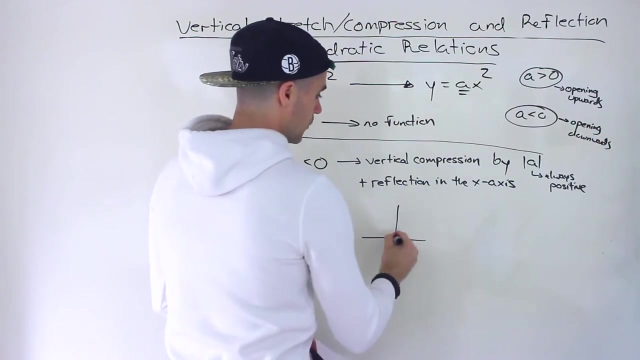 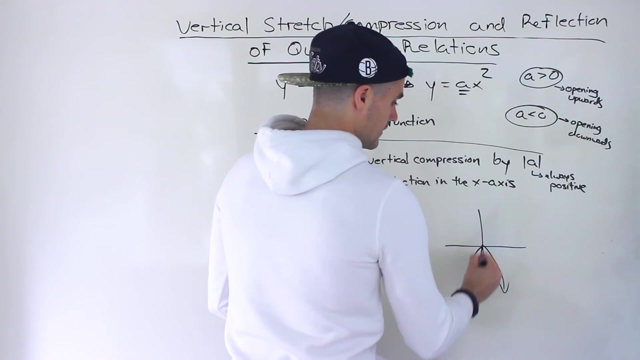 okay. but if a is less than zero, if it's negative- which is the three cases we're about to go over- then the quadratic is opening downwards- okay. so instead of a quadratic opening up, we're going to end up having quadratics that open downwards- okay, and they're either going to be stretched or they're going to be compressed. but 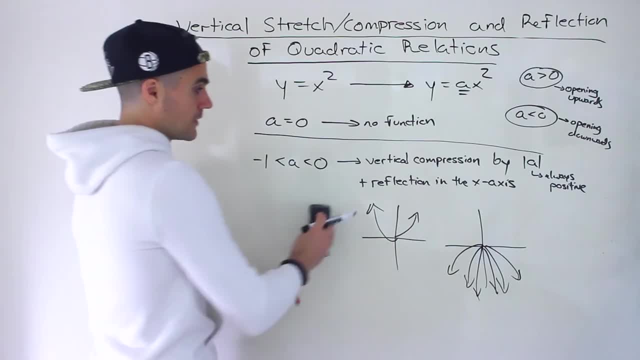 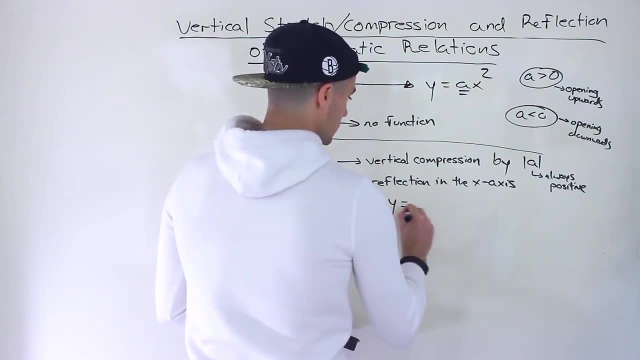 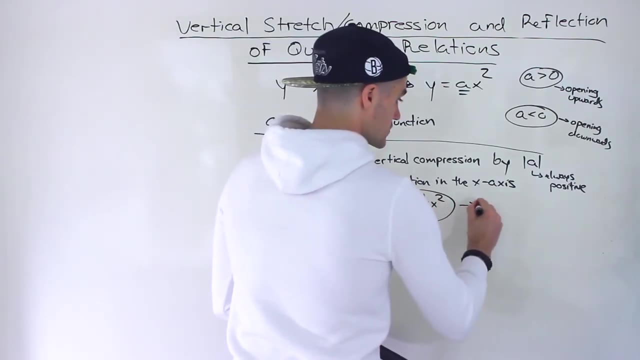 nevertheless, they're going to be opening down, and so the way this particular case would look. so, for example, y equals negative one over three, x squared. if they ask you to state the transformation of this like we said, there's a vertical compression by one over three. okay, there's. 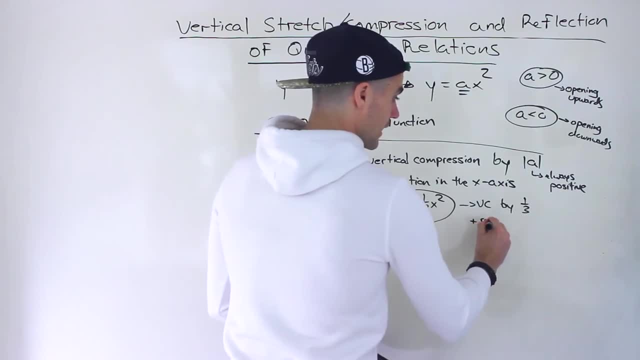 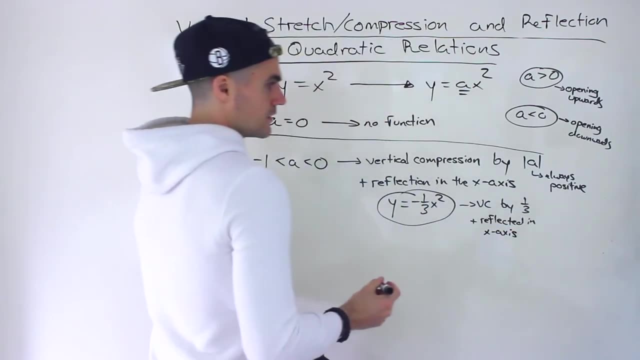 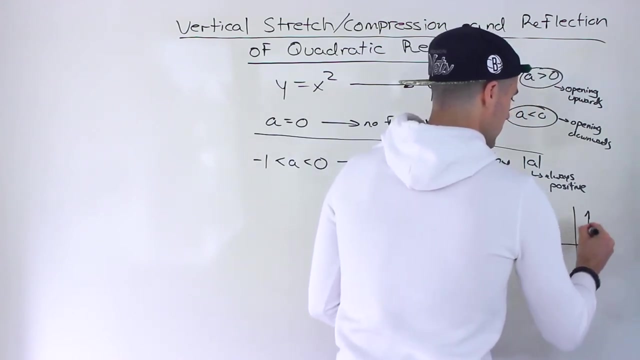 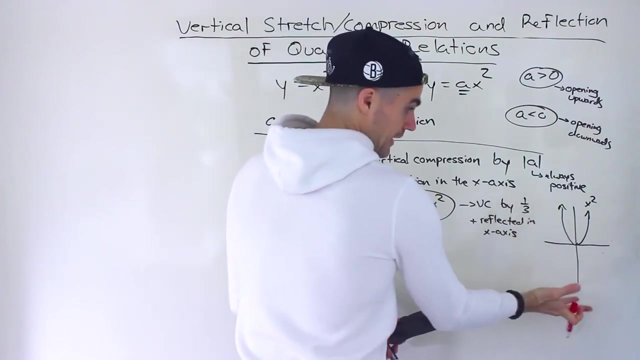 still a compression here. but we also have to say it's reflected in the x-axis. okay, and the way that is going to look. if we have, let's say, x squared like that, that's the base function, x squared. well, what's going to happen is it's going to be reflected. so now it's going to open downwards, but it's also going to be. 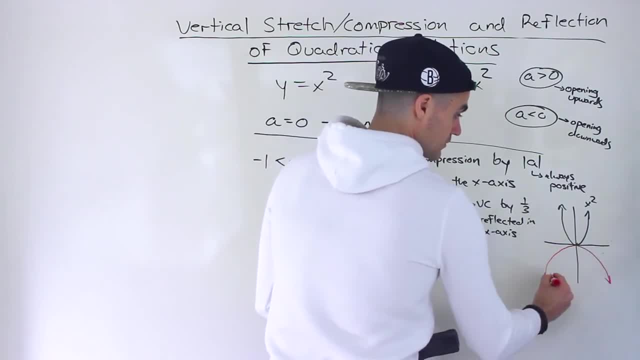 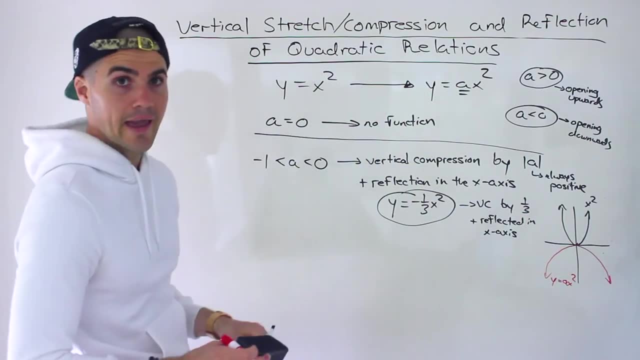 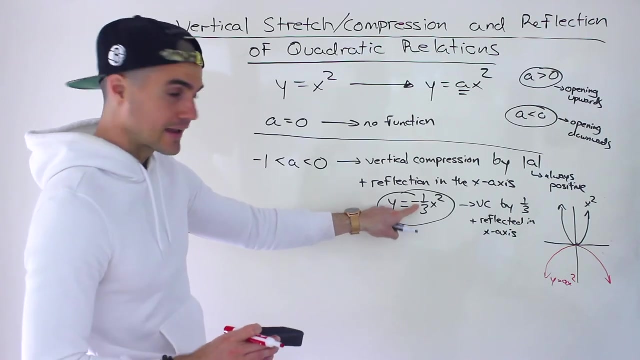 compressed, so it's going to be a wider function like that, right? if that a value is between negative one and zero- and again, be careful with your fractions- like, for example, negative four over three, that would be like negative 1.33. that's not between negative one and zero, right, that's less. 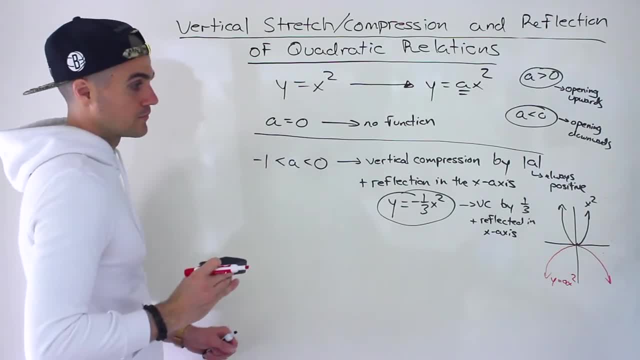 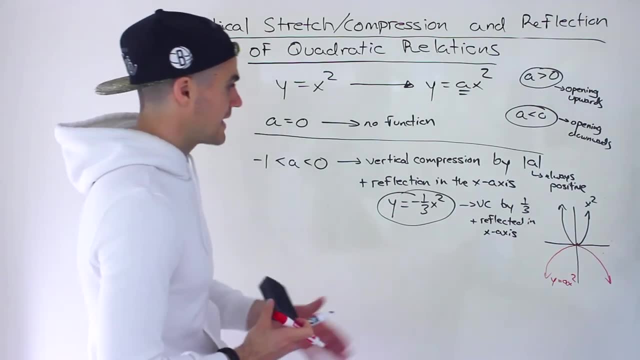 than negative one, which is a case we're going to go over in a little bit, but it's going to be a go over in a sec, so same thing applies. just be careful with these fractions over here, right? so if you see a negative, it might be useful to just write reflected in the x-axis and then just forget. 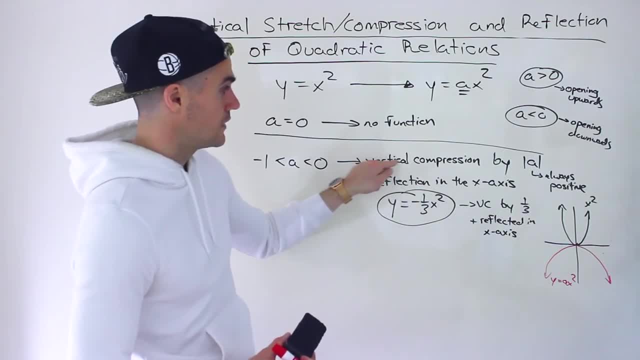 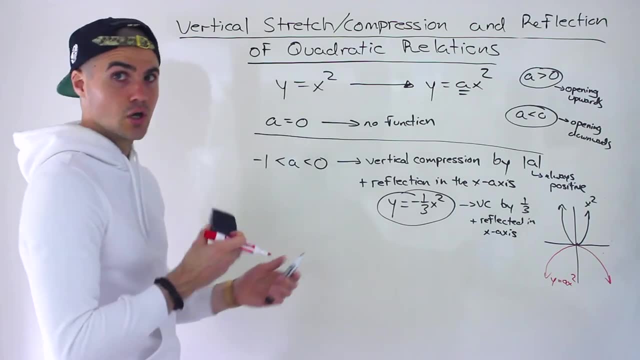 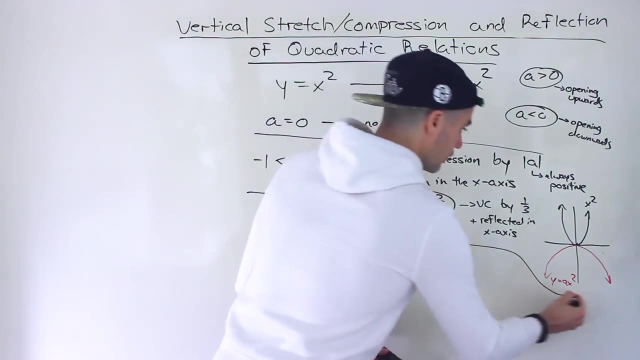 about the negative and then just treat it as a positive there, and then you could write that same transformations that you would write if it was positive, that vertical compression or stretch. all right, so that is the next case. now the following case after that is pretty simple. it's if a is equal to negative one. 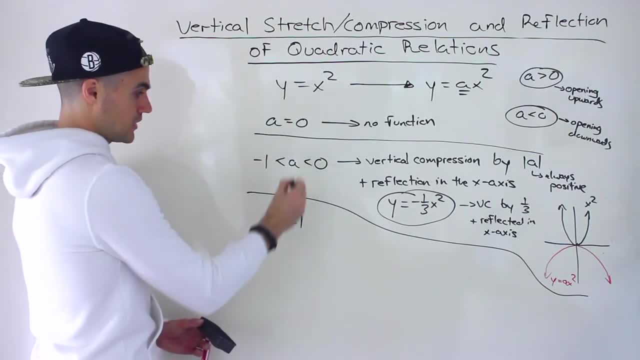 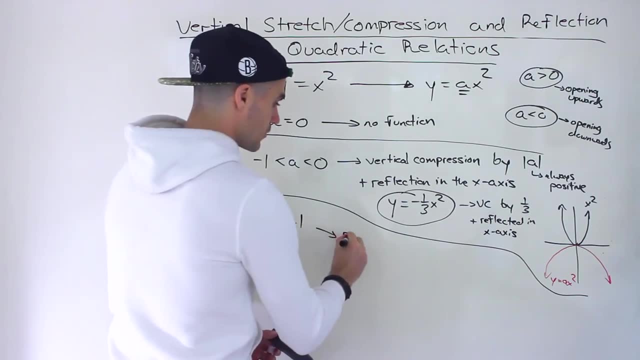 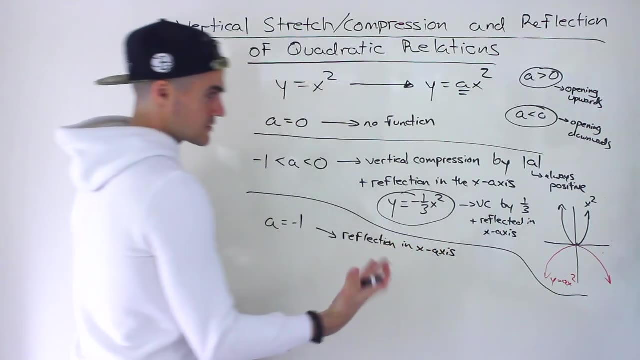 right here. it's between negative one and zero. the next one is negative one. this one's really simple notice. there's no vertical stretch or compression, but there is a reflection in the x-axis. so remember, when a was one, there was no transformation. we just ended up with that. 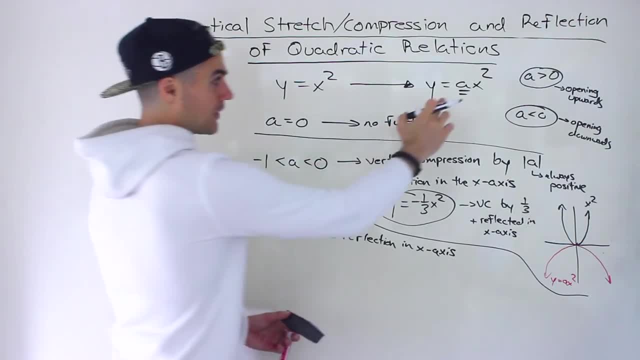 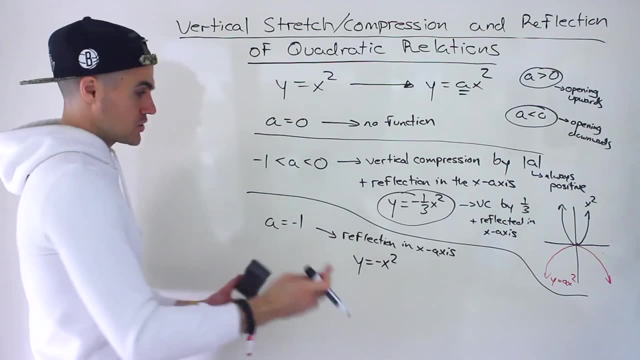 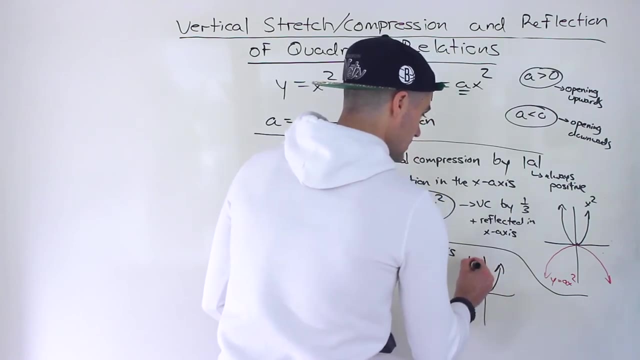 same base function, x squared. but if it's negative one now, we'll have negative x squared and even though there's no vertical stretch or compression, there's still a reflection in the x-axis and the way that looks. very simple, we got x squared like this. then a value of negative one or negative x squared is going to have that same shape, but